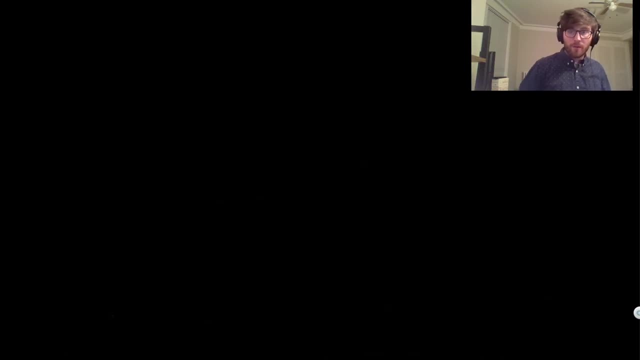 ago, when we proved this characterization of what it meant for a set to be a well-ordering. Remember our set's well-ordered if, and only if, there's no infinite descending sequences. And in one of the directions, namely the one where we assumed, our set wasn't well-ordered. 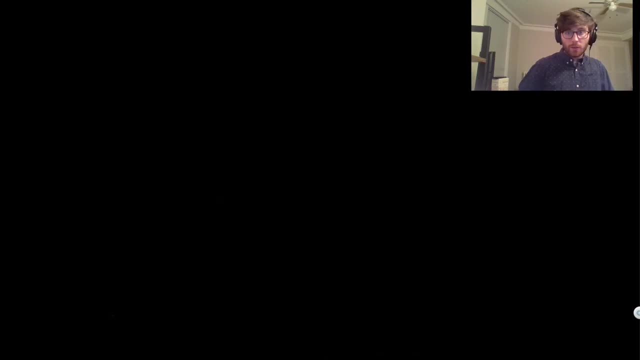 and constructed an infinite descending sequence. we constructed the sequence by recursion or we constructed it recursively, And this theorem is going to be the justification for why we were able to do that. But it's more general because that was just recursion on the natural numbers. but this works for any well-ordered sequence. 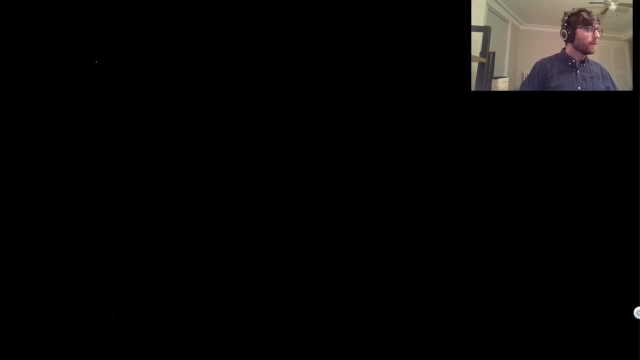 Well-ordered set. What we'll need first is a definition. So a function or f is a partial function. f is a partial function, A partial function From a to b. Well, what would it mean to be a partial function from a to b? Well, you are a function. 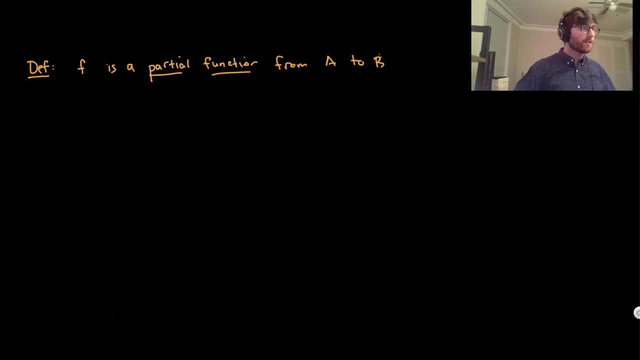 but your domain might not be all of a, It's just going to be some subset of a. So if there's some subset, a prime, such that f is actually a function from a prime, then f is a partial function from a to b. And the way that we might denote that we 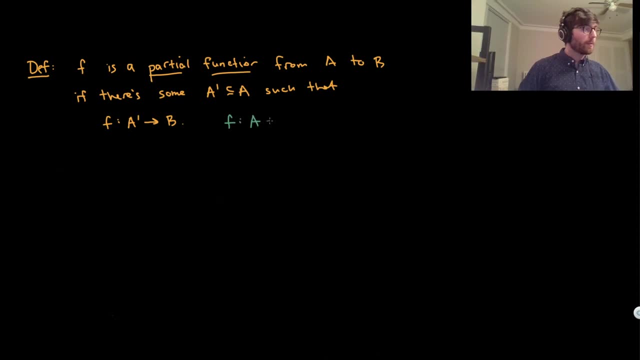 might denote this: f is a partial function from a to b. We'll write the right arrow, but with only the top hook, I guess. So f is a partial function from a to b. Well, if it's a function, whose domain where it's, if its domain is some subset of a, And if 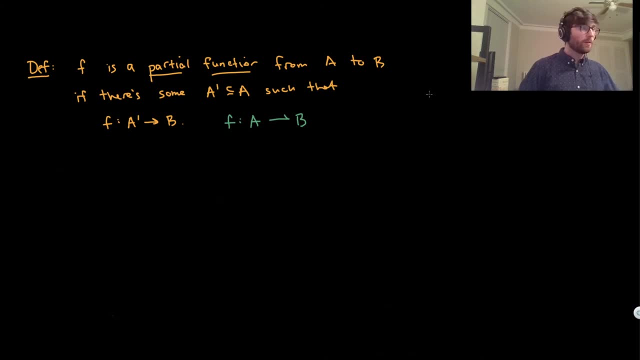 we were to kind of maybe think of the graph of something like this. let's say that we could graph it. What would it look like? Let's say that a was right here and this was b. Let's say that a prime was this green stuff right here? Maybe our partial function looks something. 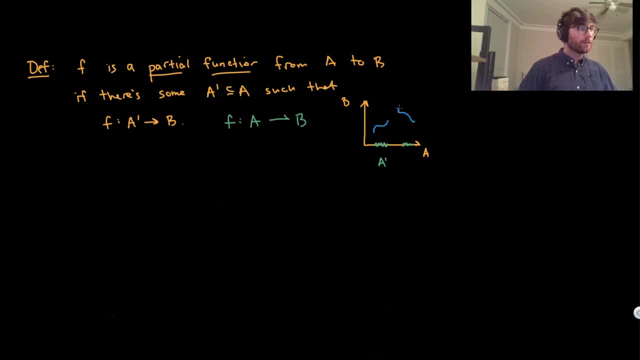 like this: Okay, I guess this fails the vertical line test, but let's pretend that it didn't. So this might be a partial function from a to b. So that is what a partial function is. What is going to be the statement of the 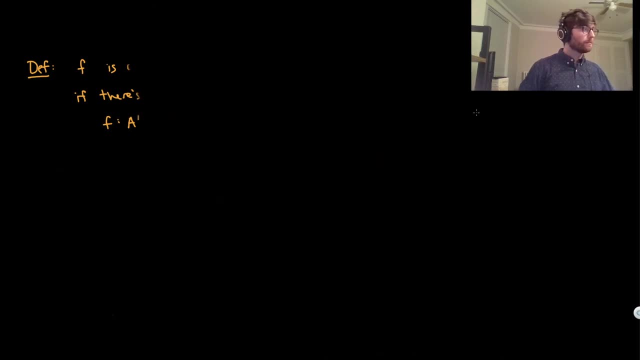 of the result We're going to prove. here's our theorem. This is going to be for recursive definitions. So here's the statement: Let a be a well-ordering be, some set, and let's assume that f is a function from a times p into b. 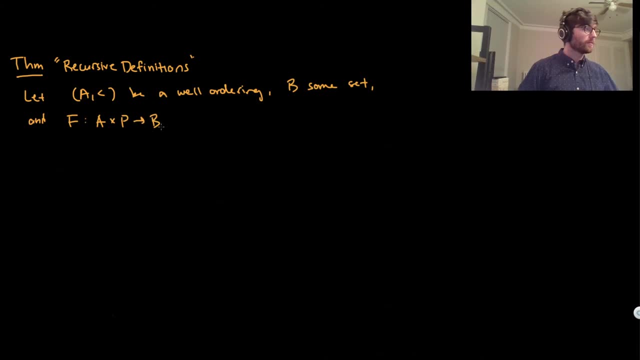 Now I didn't tell you, I didn't say what p was. So we have a well-ordering a set b and this function, big F, where what's p? p is going to be all partial functions from a to b, All partial functions from a to b. 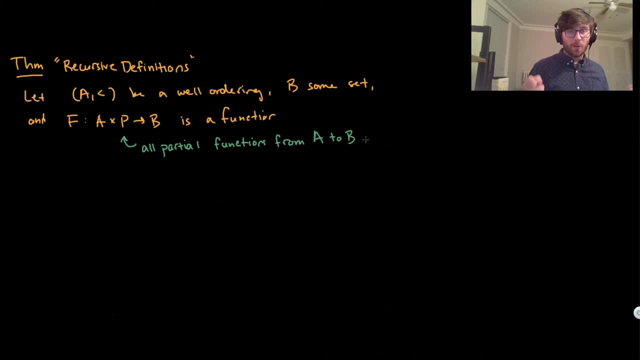 Okay, now what just happened? What is f supposed to be? Well, b is a function from a to b, So big F is supposed to be the rule that we use to kind of generate our recursive sequence or function. So if we're defining something recursively, we normally have a rule that tells us if we're given all the previous terms. 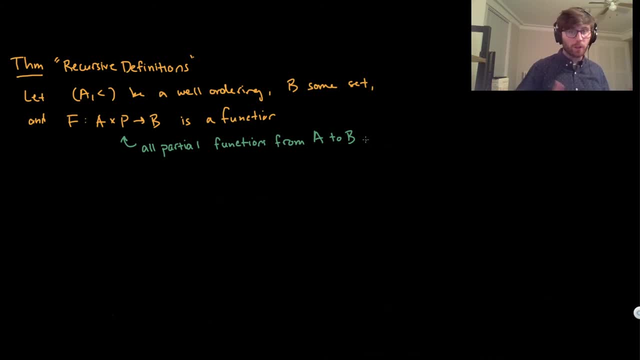 how do we get the next one? This big F is supposed to be representing what that rule is. So this is supposed to be the rule. Big F is the rule. Big F is the rule. And then what's the conclusion Of this theorem? 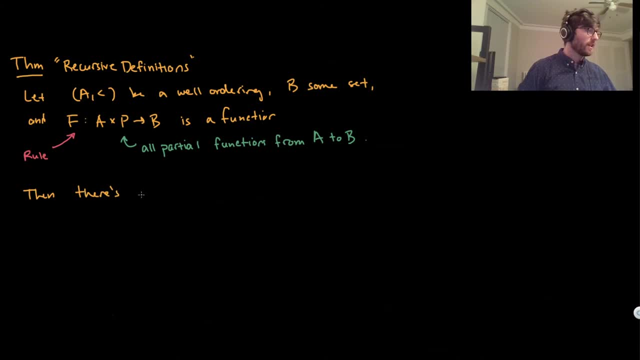 Then there's a unique function, big G, A unique function, big G, And this is going to be a function from all of a to b. such that, what is true? Well, such that, for every single value, y in our well-ordered set a. 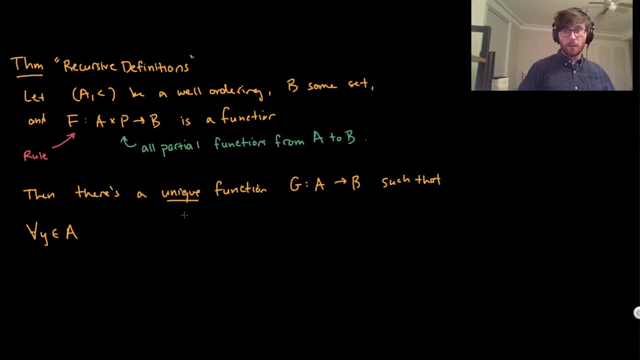 well, g is supposed to tell us what we're supposed to be able to figure out, what g of y is? Well, this is supposed to be the y-th recursively defined element. How do we figure out what that is? Well, we're going to have. it's going to be what the rule tells us to do when we have access to all the previous elements. 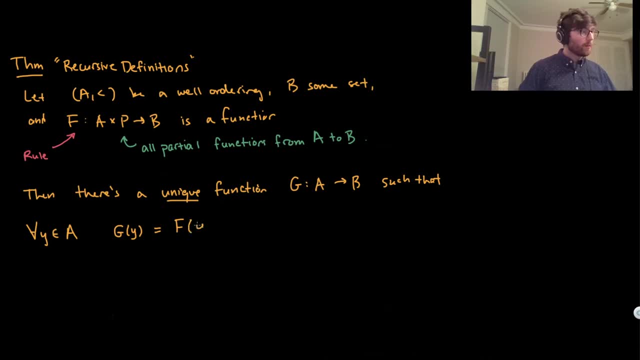 So this is going to be what our rule F tells us to do. when we have access to y, right, If we're plugging in y, we should be able to use it as a parameter. And what's our partial? Our partial function is going to be g, restricted to all of the previously defined values. 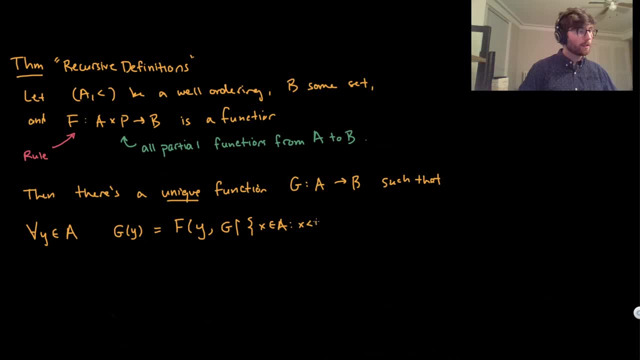 So it's g restricted to all the predecessors of y. All right, so let's say that again. So we have our big F, that's our rule, And what the input, what the domain of our rule is, is going to be our set a. 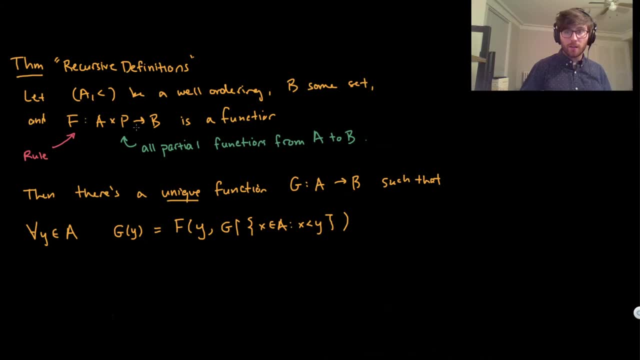 Because if we're plugging in, if we're trying to figure out, say, what the 20th recursive element and our recursive, our sequence is, we should be able to use 20 as a parameter And this set of partial functions here, from a to b, that's supposed to represent all of the previously defined information. 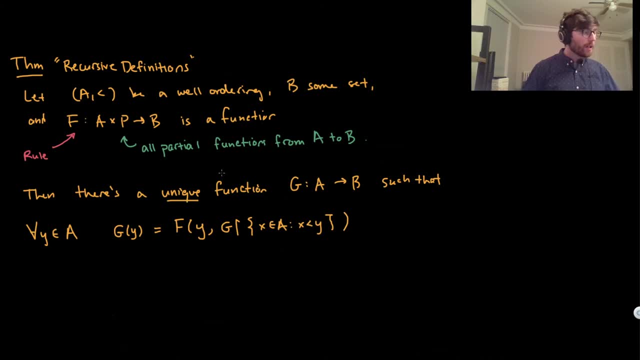 And what's the conclusion is that there's a unique function, big G, such that if I plug in any value in a, so y. so if I want to figure out what g of y is, its output is going to be what the rule told us to do, assuming that we had access to all the previous information. 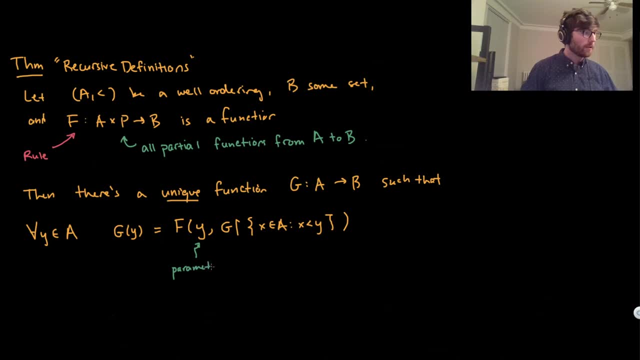 So this is our parameter y. You can think of this as a parameter. And what is this? this is this. this is encoding all of the oh, this is all of the previously defined values. So just remember, if you have a function and you this, this, this notation here means that we're taking the function and we're restricting, we're restricting the domain to this set here. 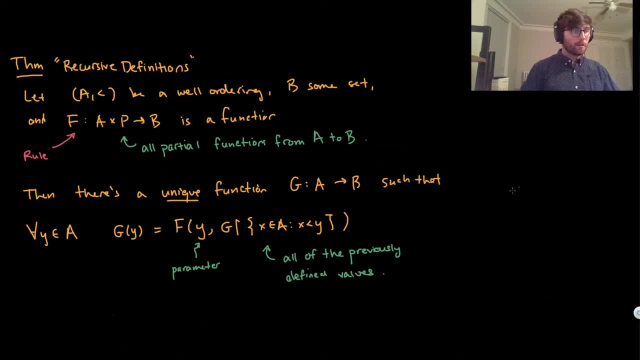 So I'll write it over here. So g restrict it to this set. Well, this is the function g with domain this set. And why is this function g in our set P right? The right coordinates here are supposed to be in P. 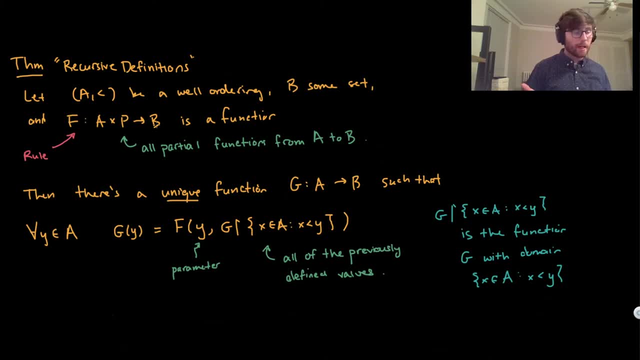 Well, we're assuming that we have this function g already, And if we have this function g, it's a function from a to b. So if we restrict the domain to any subset of a, it's going to be a partial function from a to b. 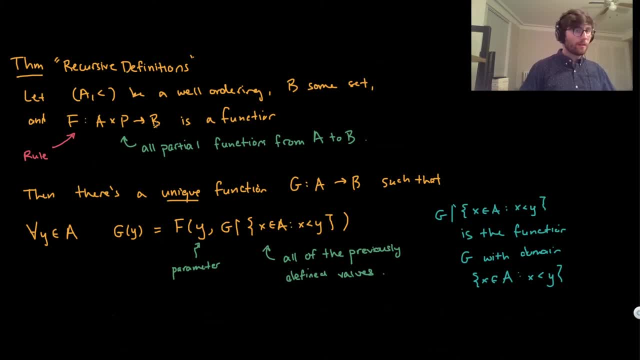 Okay, so that's the statement of of of the theorem. This is I. when I saw this for the first time I knew what recursion was And I knew how to kind of give recursive definitions, But for some reason I thought this was. I found this kind of really technical. 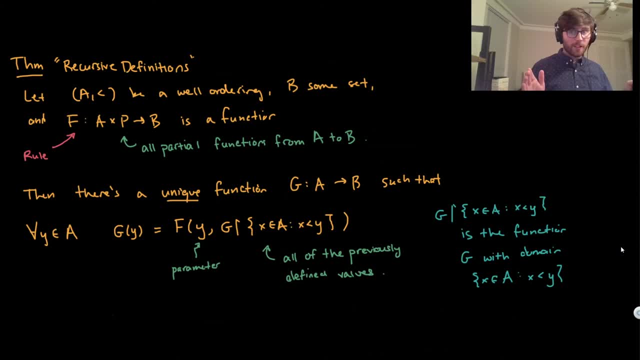 So let's maybe give an example Before we give the proof. let's give an example of, say, how to recursively, of let's define the Fibonacci numbers recursively, And let's do it in such a way where we kind of are making the, the, the setup look. 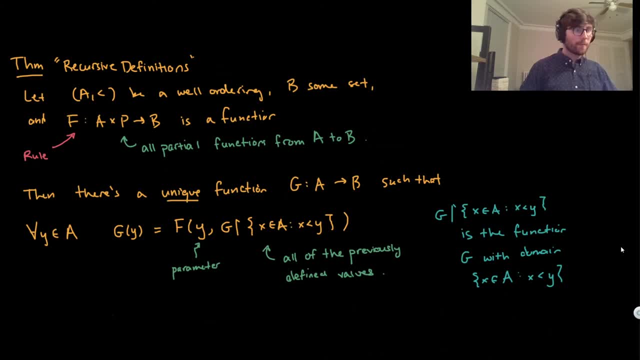 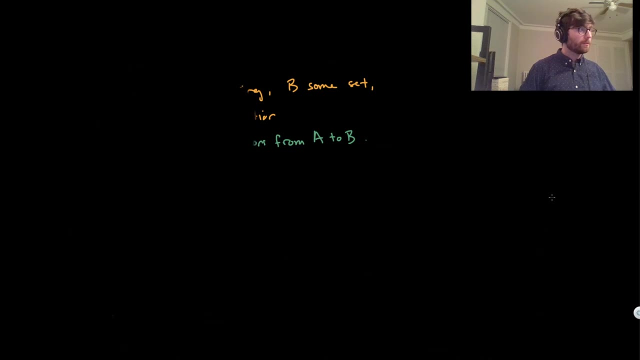 like the hypothesis of this theorem and see what happens. So we're going to give an example. Let's define the Fibonacci numbers. So what's the setup? Well, we need to say what our well-ordered set is, And in this case it's going to be omega with the membership relation. 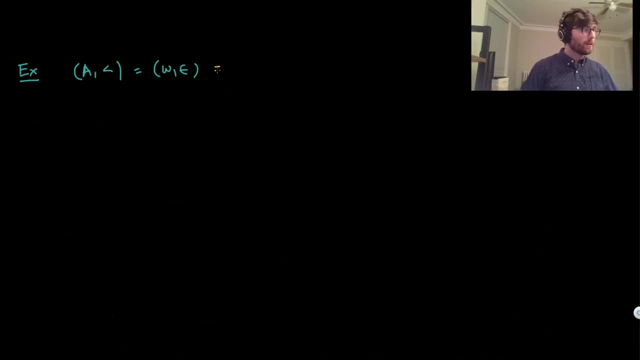 And remember well, omega is just the natural number, so we can kind of really just think about this: This is just the natural numbers, with the less than we're doing. And so in the statement of our theorem we needed our set A. 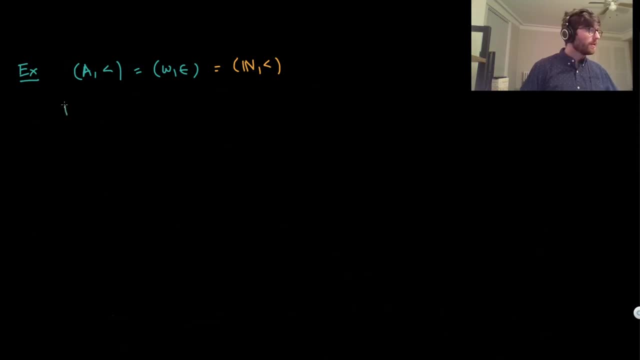 but we also needed the set B, And the set B is going to be omega union. this extra set, Let's call it error. So what is this term? This is just any set that's not in omega. Now, remember, in the hypothesis of this statement of our recursion theorem. 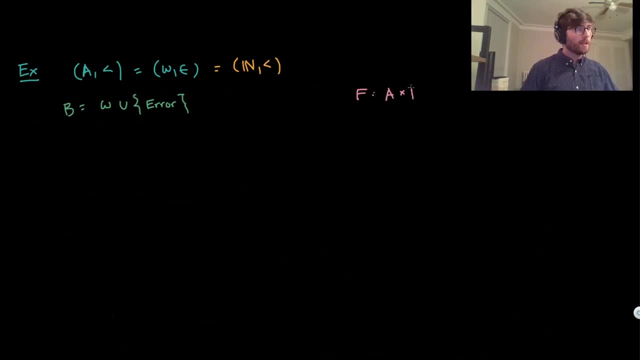 we have this function big F from A times P into B, And what's about to happen is- or why do we need this error term? Well, P is all partial functions from A to B And in this case it's going to be all partial functions from omega into this set B. 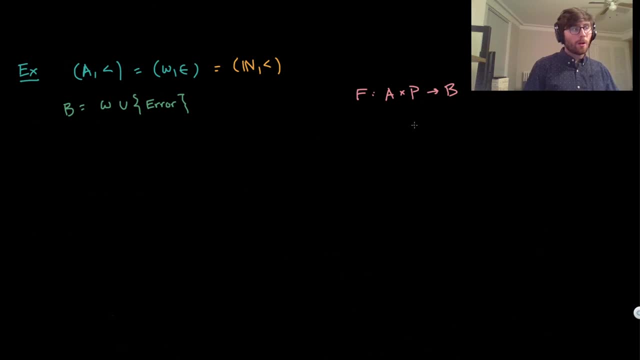 omega union this additional error set. Well, if we're going to give a recursive definition, we don't need access to all the partial functions. We just need access to the partial function of the previously defined information. So this function F is going to give us a lot of unnecessary information. 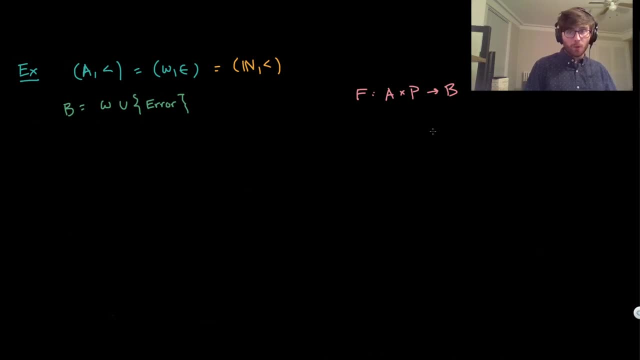 And so what we're going to when we give this definition of our rule, we're going to have to say what we do when we kind of our two inputs are either incomprehensible, or it doesn't make sense, Or just if something crazy happens. as an input we just want to output error. 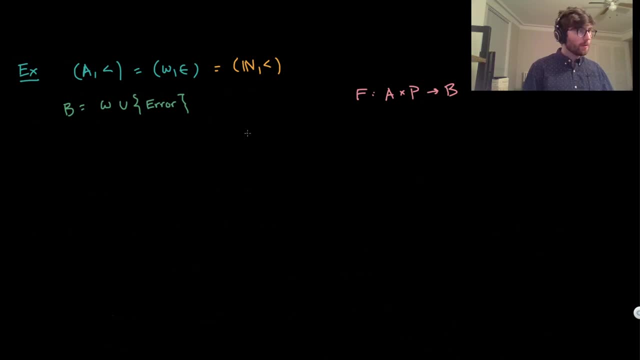 We don't want to think very hard about it. So what's going to be the definition of this F? So we're going to try to define the Fibonacci numbers. Well, F is going to take two inputs. It's going to input a number. 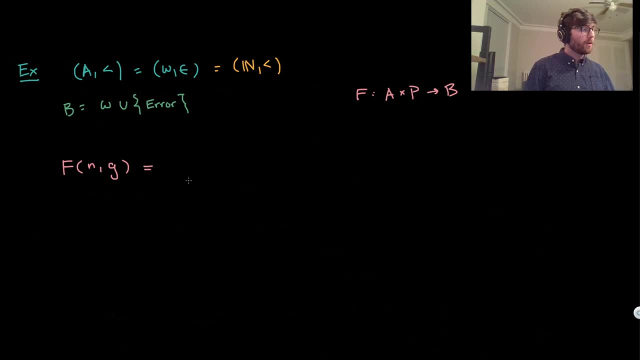 It's going to take a natural number and a partial function. And what's the output going to be? Well, it's going to depend on, it's going to be a definition by cases. Well, if n was zero, then what we're going to output is zero. 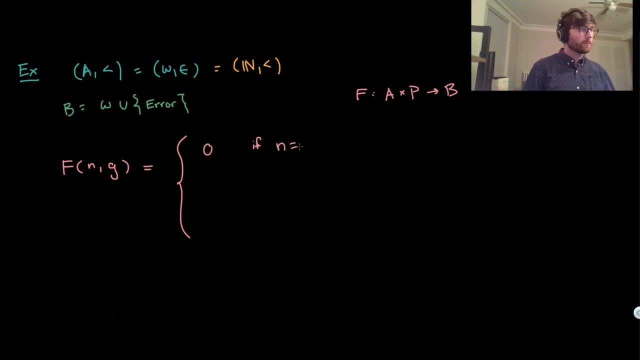 So if n is zero And if n was one, then we're going to output one. Those are the first two numbers in our in the Fibonacci sequence. And what's going to happen when n is bigger than or equal to two? We're going to output one. 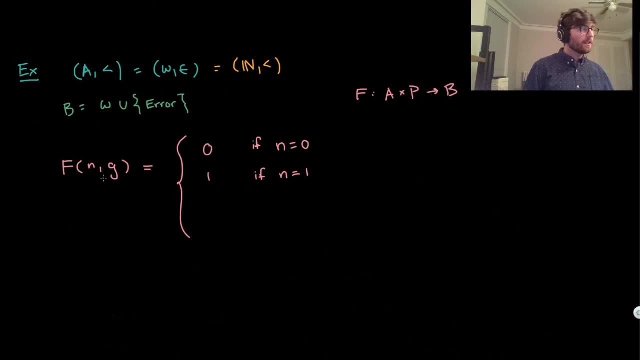 We're going to output the sum of the previous two values, And in this case we're going to. g is supposed to be representing all of the previously defined values. So what we're going to do is we're going to output g n minus one plus g n minus two. 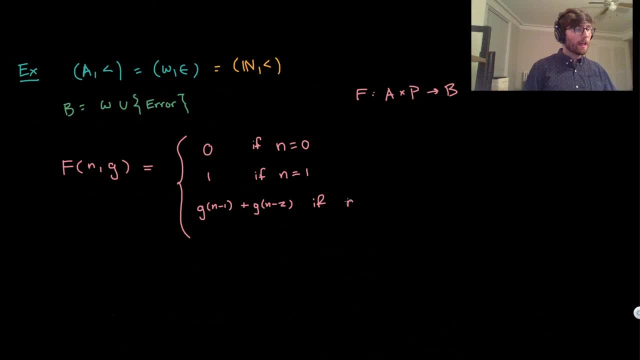 If what happens? Well, if n has to be bigger than or equal to two, g can be any partial function. So we just want to make sure that, if we're doing this, we want to make sure that n minus one and n minus two are both in the domain. 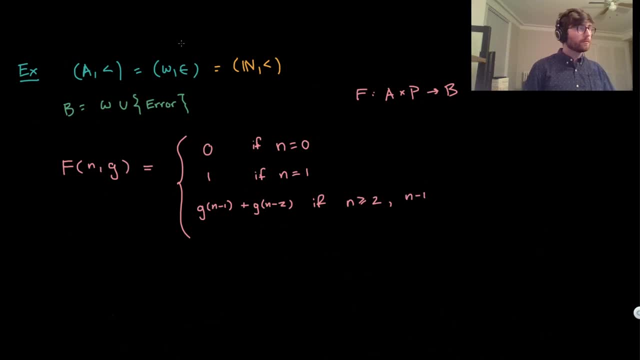 Of g. So n minus one is in the domain of g And n minus two is in the domain of g, And the other thing that we need is that g n minus one and g n minus two we shouldn't have, they shouldn't be the error term. 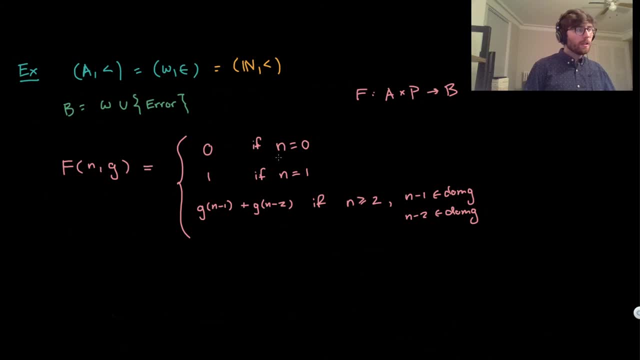 So let's say that, if so, again e can be any. it's going to be the set of all partial functions From a to b. So maybe g would have, maybe n minus one and n minus two are both in the, are both in the domain of, of our function g. 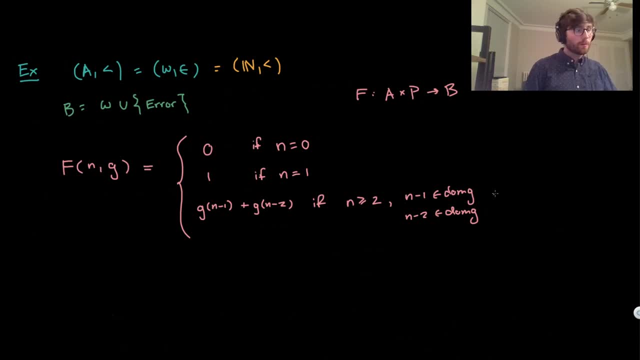 But maybe the output was the error term And if that was the case, what we're going to do is we just want to make sure, in this case, that g n minus one and g n minus two are not both the error term, So they're both not the error term. 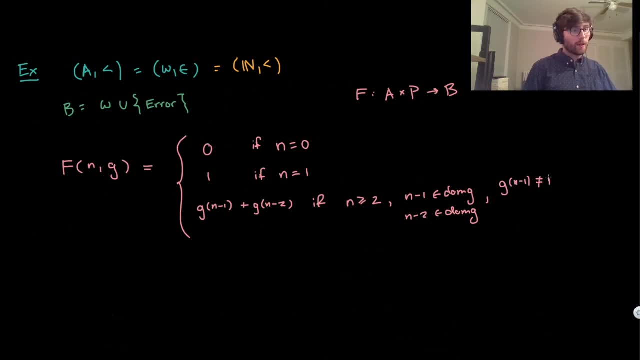 So g n minus one is not equal to error And g n minus two is not equal to error. If we're in a situation like that, then well, this definition makes sense: g n minus one and g n minus two are both going to be natural numbers. 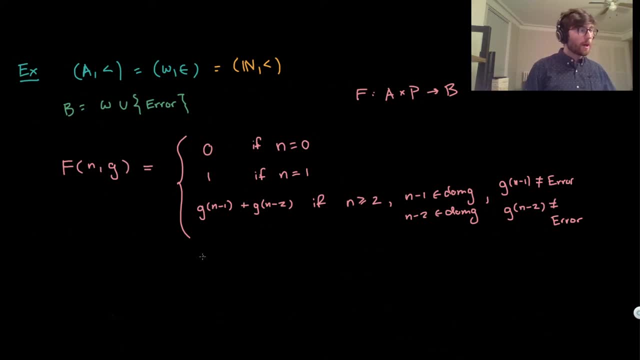 And we're going to be able to just add them up, And what we'll do otherwise is, if we're not in any of these cases, we're just going to output error. We're going to output error otherwise, Okay. so what does the theorem 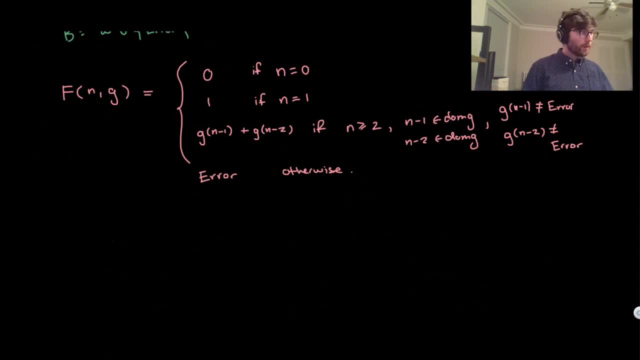 What does this theorem do? What does this theorem tell us? This theorem tells us, so the recursion theorem, what it's going to give us Theorem. It gives a unique function, g, And this is going to be from omega n to omega union, the error term. 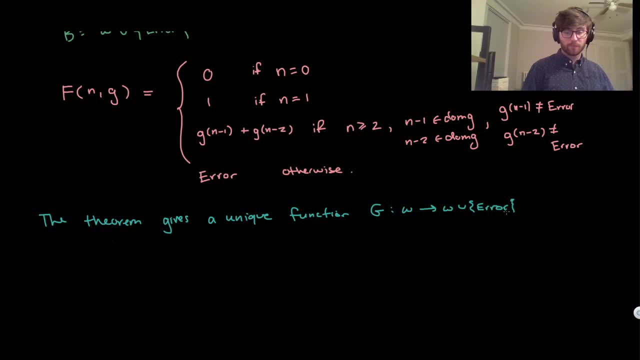 And this is going to be from omega n to omega union, the error term, such that for each natural number, well, g of n is going to be f of n, And then what's going to be our partial function? it's going to be g, restricted to all of the natural numbers that come before it. 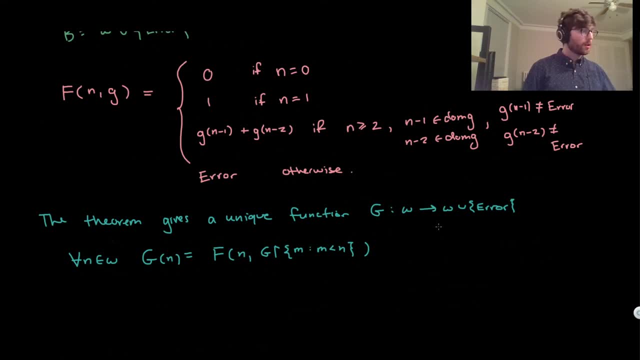 So this is what the conclusion is, And then what's going to be our recursion of this theorem? Now, there are some things that you can actually show By induction. if you did an induction on n, So by induction on n You can show that this function g is actually never going to output error. 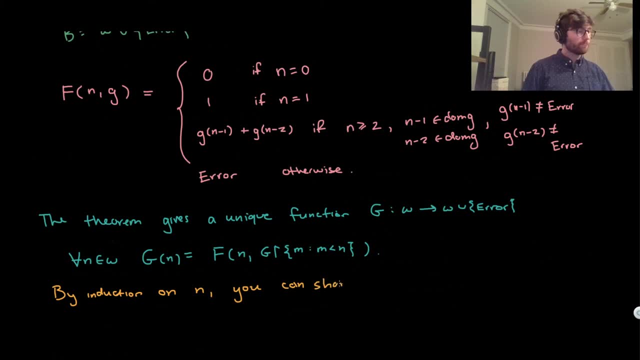 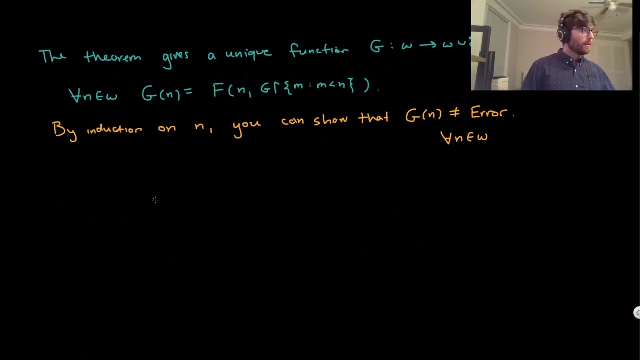 So Okay, Okay, Okay, Okay, Okay, Okay, Okay, you can show that that g, n is never equal to is, is never equal to error. so you can just show that by induction on n and well, if you kind of unravel what all this is saying, what we're gonna get is: we're gonna get the following: so 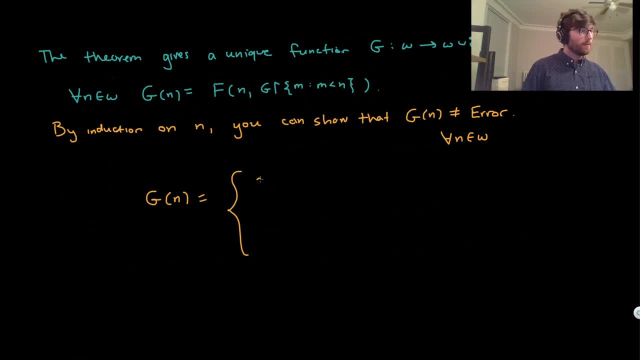 g of n is going to be equal to well, it's going to be equal to zero. if n is equal to zero, it's going to be equal to one. if n is equal to one and if n is bigger than or equal to two, what we're gonna get is we're gonna get g of 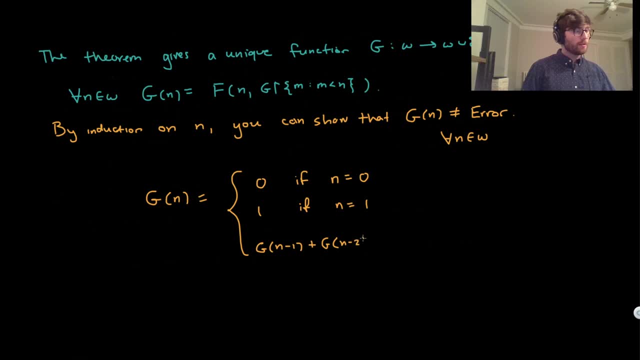 n minus one plus e of n minus two, and is bigger than and. so okay. so so that's what this theorem is giving us at the end of the day. now, how do we actually compute this in practice? in practice, what we're going to do is we're we're not really computing all of g at once, we're just computing. 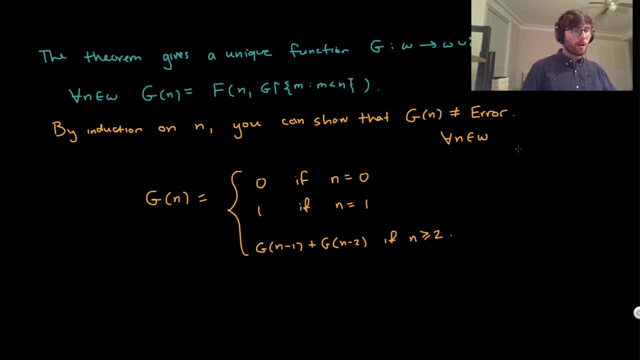 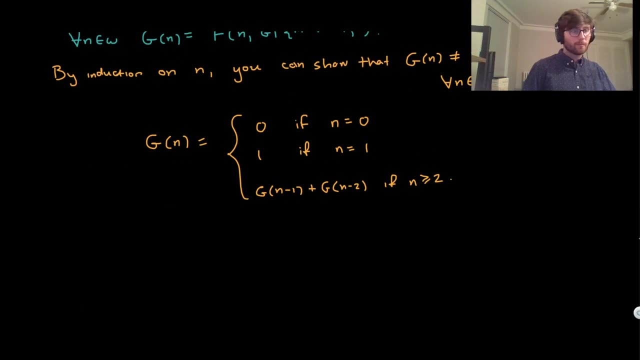 kind of these uh like approximations of what g are. so in practice we don't actually compute g, we compute approximations of g. maybe we'll put some more space done in practice. in practice we don't compute all of g at once, all of g at once. 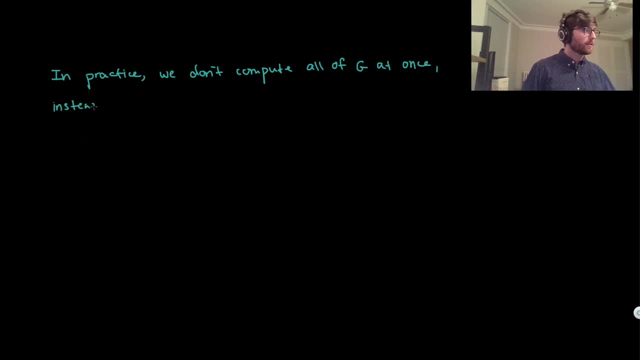 instead we compute approximations of g. approximations of g. so what do i mean by that? so in in our fibonacci example, well, if we want to figure out, i guess, what our first approximation is, so what we get when we plug in 0. well, that's just going to be say 0. 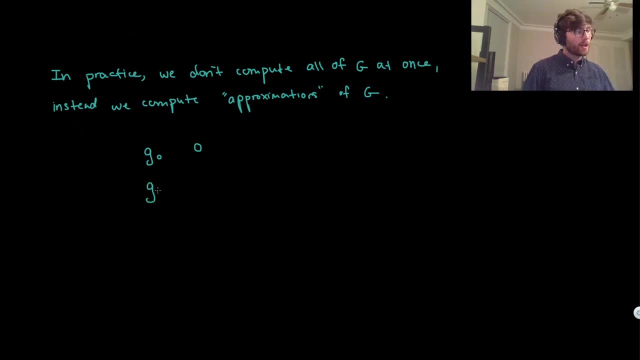 if we want to figure out what the next approximation is. well, we're going to have access to 0 already, and then we we want to input 1 and we know we're going to get 1. what about for the next approximation of g of n? we're going to use 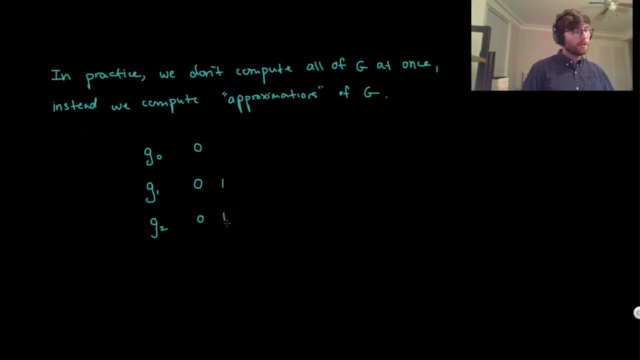 the next approximation, we have access to the previous two values, and what we're going to get to get to the next one was we're going to add the previous two values together, so we're going to get one again. what about for the- uh, i guess, the fourth approximation? we're going to have access to all. 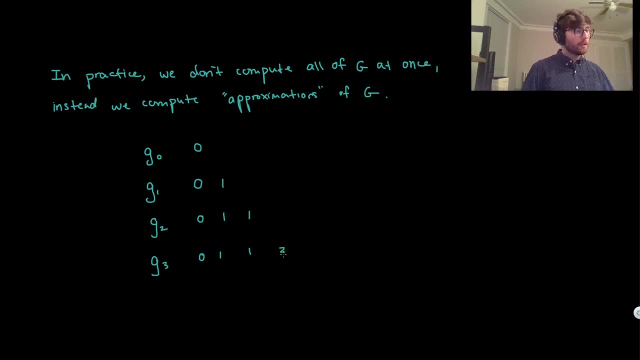 the previous values and to get the next one, we're going to add the two values. what i'm trying to get out here is that we're not actually ever, uh, uh, following this procedure. we're kind of defining g, but we're defining g by just kind of defining all a bunch of approximations of what g is and if 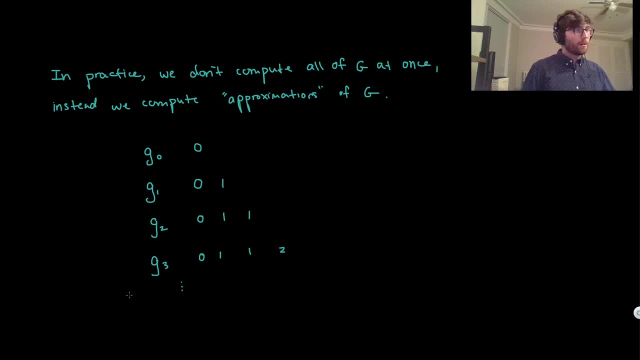 we say wanted to figure out what the 400th, uh, uh, what we get when we plug in 400 into g. we're computing the first 400 approximations of this thing and then using that to figure out what the next value is. so we can think of all these things as partial functions. so this is maybe what i what 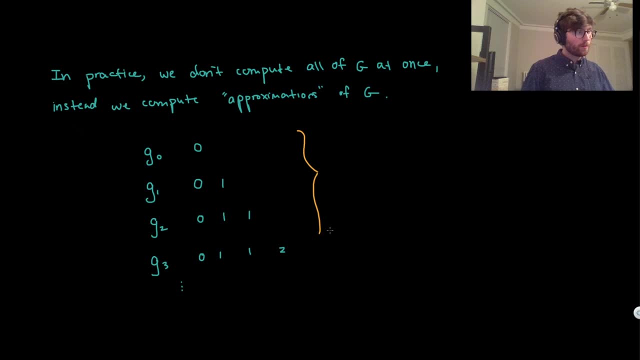 i'll stop at in this video and then we'll give the formal proof the next time. but all of these are partial functions, so each gn is a partial function from well, in this case it's going to be from omega, uh, uh to omega, but generally it's from omega into b. 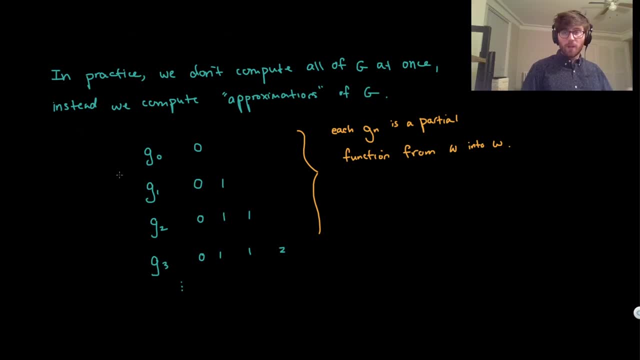 and what's going to be the uh, all these are approximations of our function big g. what's going to, how are we going to use all these uh, uh, what? what we're going to prove next time is that there's always these approximations of our function g, and then what's going to be the function g that we 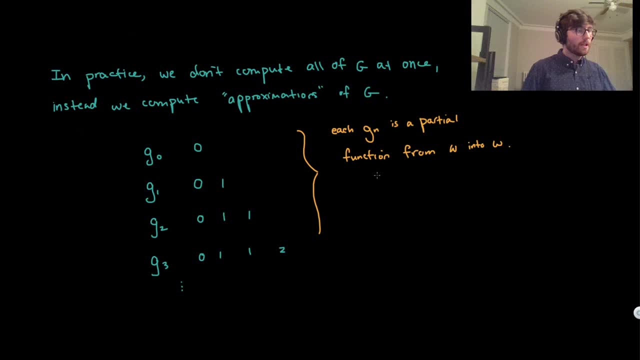 care about, it's actually going to be the union of all of these gns. so, uh, next time, what's the idea of the proof? at the end of the day, idea of the proof is that our function g is actually just the union of all of these values. 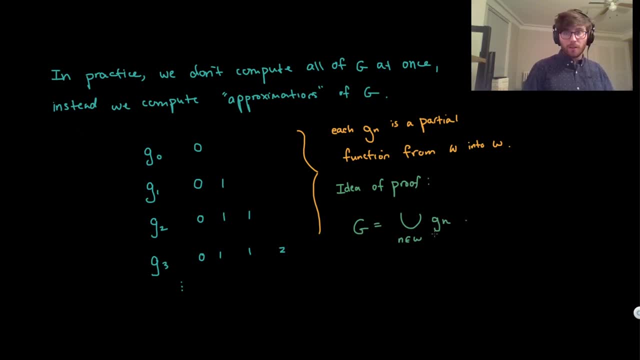 and just to kind of digest what this means. what is a function kind of set? theoretically it's a set of ordered pairs, and these are all sets of ordered pairs. we could union them all together and because they're kind of coherent, right, the, the, the input for all these partial functions. 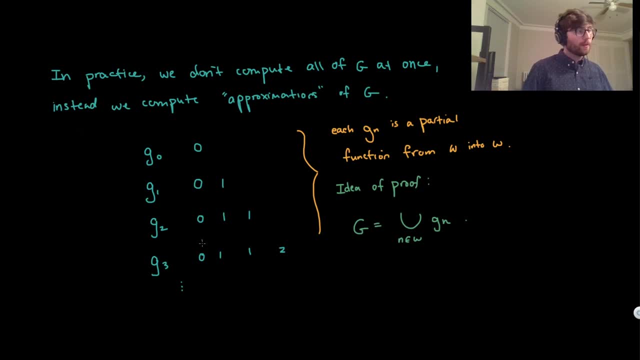 say, when we uh look at the value, and if we plug in zero into any of these, into any of these partial functions, we're always going to get zero. if we input uh two into any of the approximations after g0 and g1, we're always going to get one. these kind of functions are all extensions of each other, so 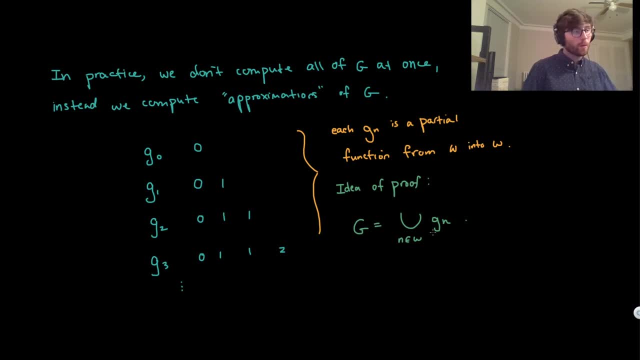 if we take the union of all of them, we're going to get a new function and we we're going to show that this, the domain of this new function, is going to be all of a, and that's going to be exactly what, uh, our function, and i guess we'll have to do some, some more stuff to make sure it all works out. 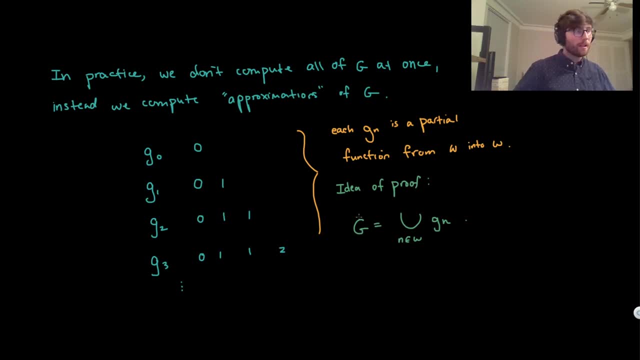 but this is going to be exactly our function g that we are searching for in uh, i guess from the start.